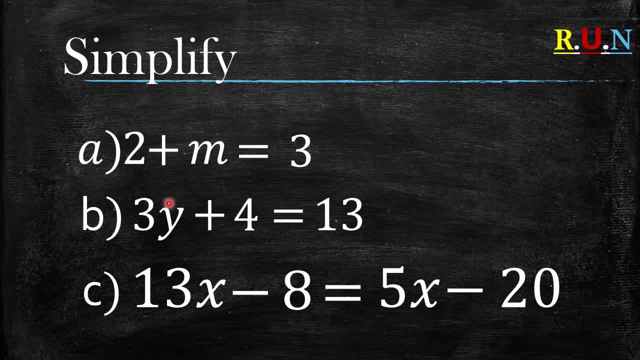 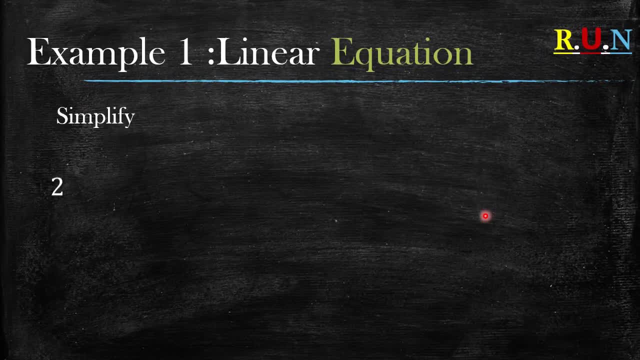 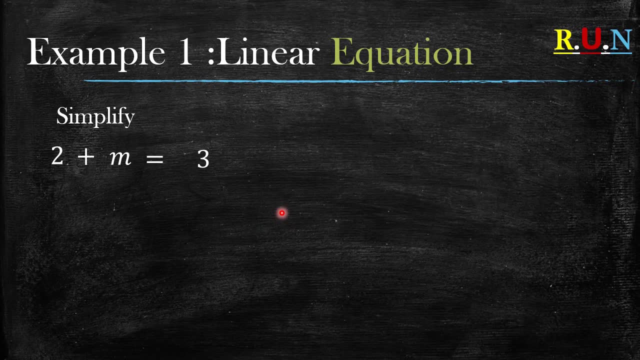 we're going to be using three example questions, okay, which are a, B and C. Example number one: So what do we do when we have a question like this, for example? so one thing to bear in mind is that we want to find the variable, or to find 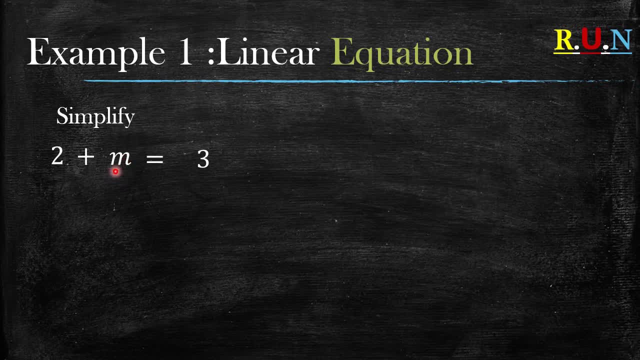 what is equal to the variable. in this case, our variable is this M. okay, what is equal to the M? because this 3 is equal to 2 plus M, but now what is equal to the M alone? okay, so now to do this, I'll be showing you two ways in which. 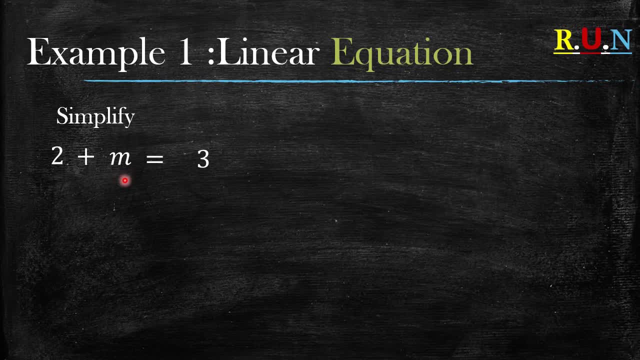 you can get the answer. So in the first way, we can do this by cancelling out this number which is with the M. okay, let's try to get the M alone. on this side the m is a positive 2, so we cancel out that positive 2 by minusing 2 on this side of the. 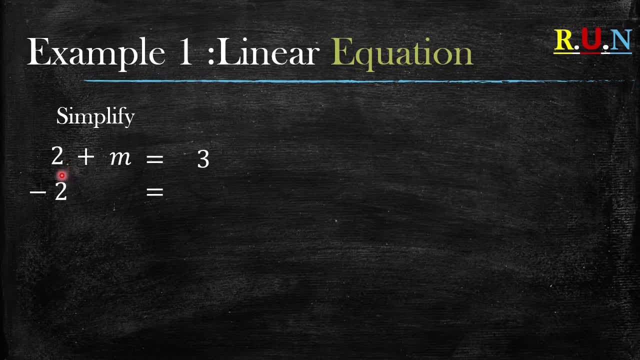 equation now, remember in algebra, or let me say in this, linear equations: whatever you do on one side, you do on the other side. now, because we minus this 2 to cancel out the 2 above. on the other side, we also have to minus a 2. okay, so 2 minus 2, what do we get? it will cancel out. so what is left? 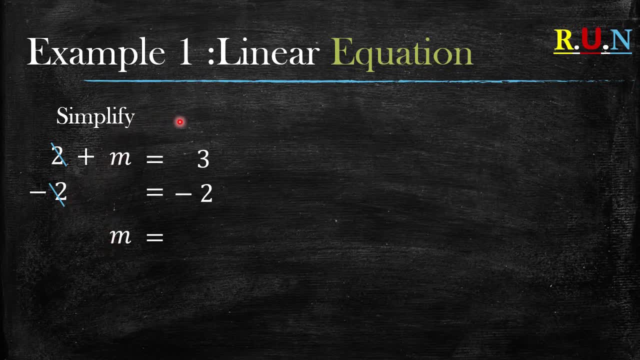 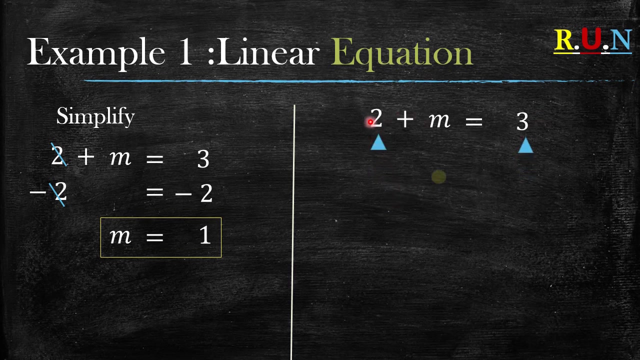 only the m is left. now, on the other side of the equation, 3 minus 2 is equal to 1, and just like that you have found your answer for the variable. so m equals to 1. okay, now you? you another way would be. so this is the same equation. i just added the triangle and the circle to make it easier. 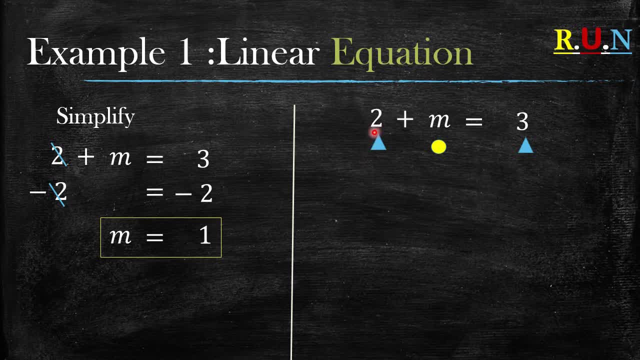 or to show the like terms. look at this 2 and this 3. these are like terms. now, this m doesn't have a like term. okay, so in this way, what we can do is take all like terms to one side. okay, so, which means this m stays alone, this side. 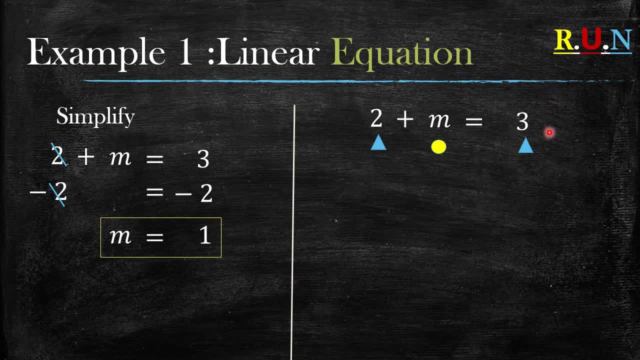 and then we take this 2 on the other side, so they can both be like terms on one side. but one thing you need to bear in mind is that each time you take a number over the equation sign or the equal sign- sorry- and then you have to change the sign. say, for example, this 2 is a positive 2. so if you 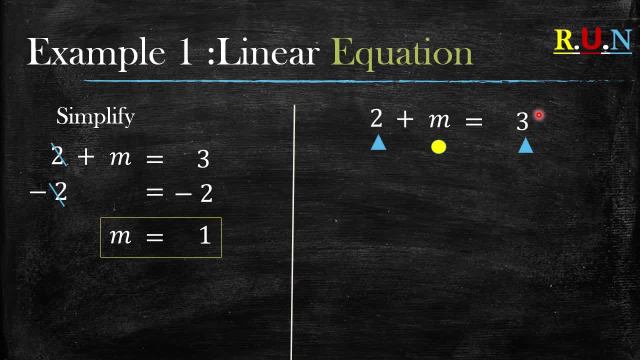 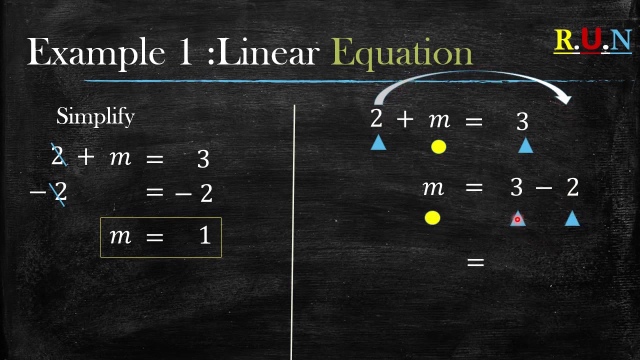 are going to take it to the other side, it will become a negative 2. okay, i'll just show you now what i mean. so this was a positive 2, but after you take it to the other side so that it can be with its like term, it becomes a negative 2. so each time, just remember that each time you move a number to the other side, the sign in front it changes. okay, so after you move it and the sign change to negative, what do you have on this side? you have the m. 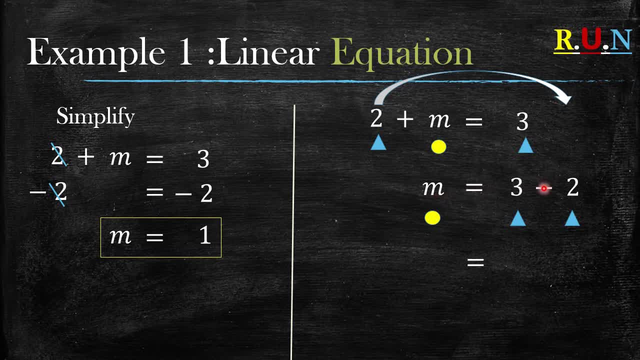 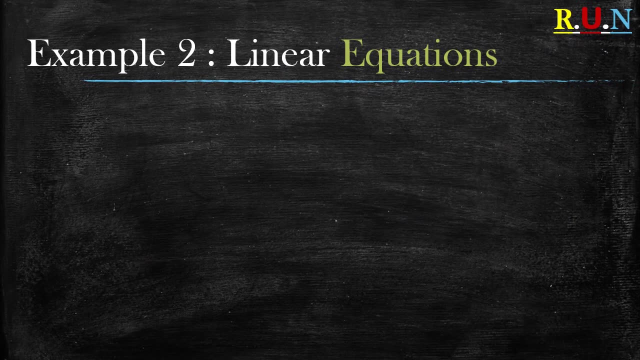 alone, which means you can actually just subtract this side, because it says 3 minus 2. what's 3 minus 2? it equals to 1, and just like that. again, you have found your answer for this side. okay, let's look at example number two. so in this example, i'm going to be using the first method. 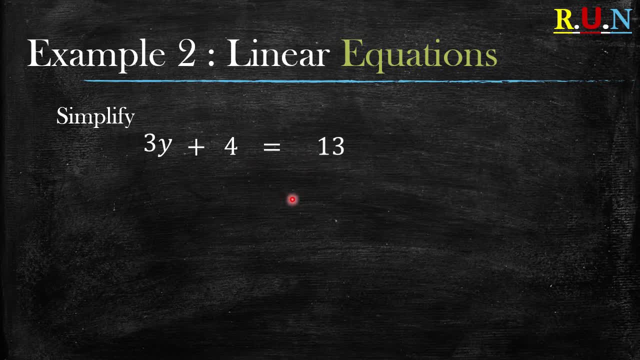 what do you do when you have a question like this and you're told to simplify, which means we want the y, this variable. so, again, the first thing would be to get this 3y to be along this side. so what do we do? in this instance? we have 3y plus 4, okay, so we cancel out this 4. how do we cancel out this 4? 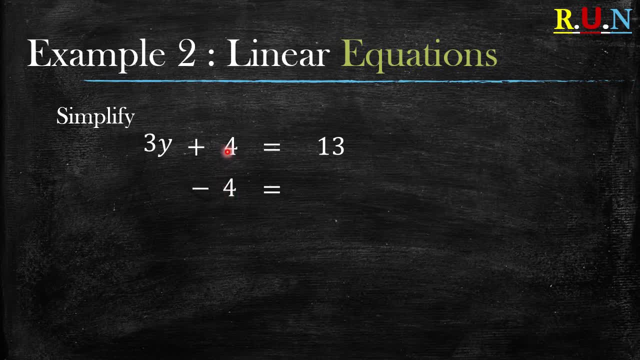 by minusing a 4. okay, now remember: when you minus a 4 on this side of the equation, you need to minus a 4 on the other side of the equation as well. good, so what's 4 minus 4? it will cancel out and. 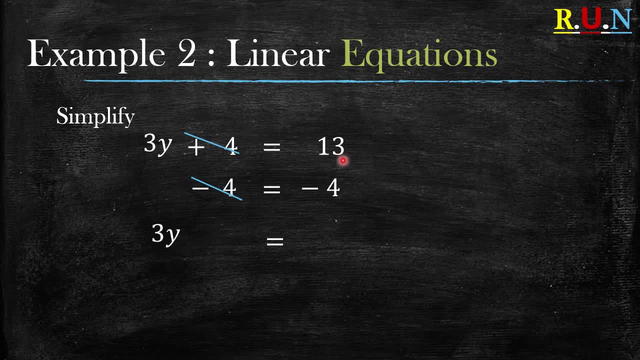 you are left with 3y. what about? 13 minus 4 equals to 9. okay, now, from here we are getting closer. it's now 3y equals to 9. now, each time you see like a 3y, this means it's multiplication, because it's. 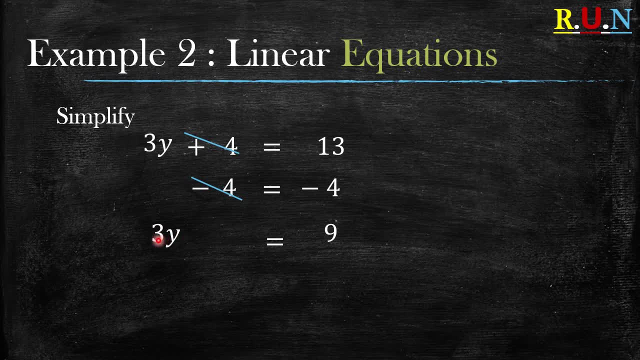 3 times 3y, because there's no sign in between there. it's just like 3y, so it's multiplication. how do we cancel out multiplication? by using division. okay, so we bring out our division lines and because we want to find y, we divide this 3y by 3. now remember, whatever you do on this side of the 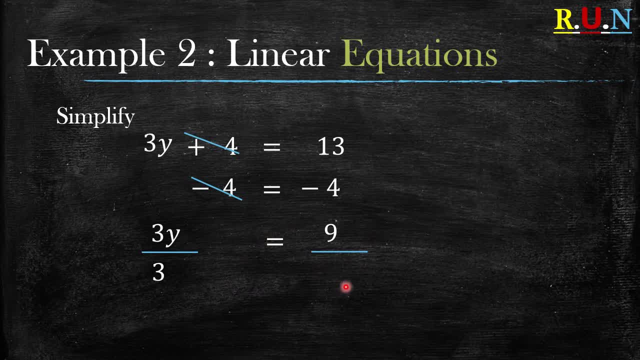 equation, you do on the other side of the equation, so we also divide this side by 3. so what's 3 divided by 3? that will cancel out. what about on the other side of the equation? what's 9 divided by 3? it's equal to 3 and just. 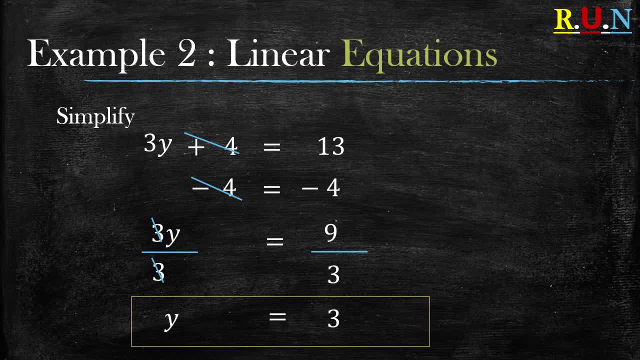 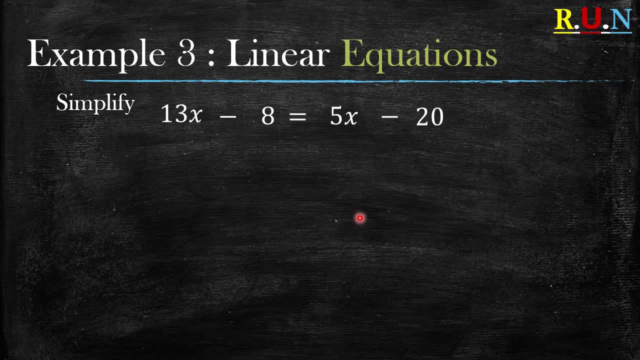 like that. we have found your answer. okay. now let's look at example number 3. so you have something like this. so what do you do? remember? our main aim is to find the x to say: what is this x equal to? now, in this question we have 13 x minus 8 and on the other side, 5 x minus 20, meaning we 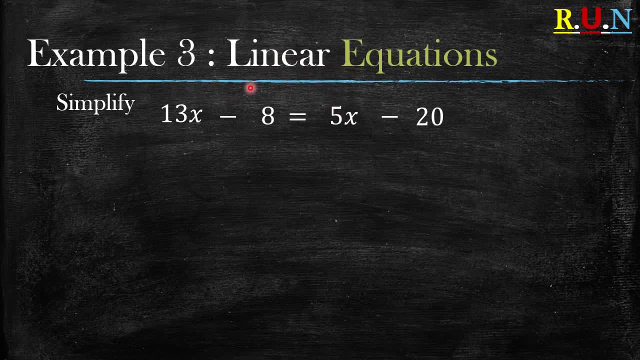 have x on both sides, okay. so what do we do? let's start with this side. so let's keep the 13x and cancel out this minus 8, or negative eight. so how do we cancel out negative eight? by By plussing a 8, negative 8 plus 8 will cancel out this 8, okay. 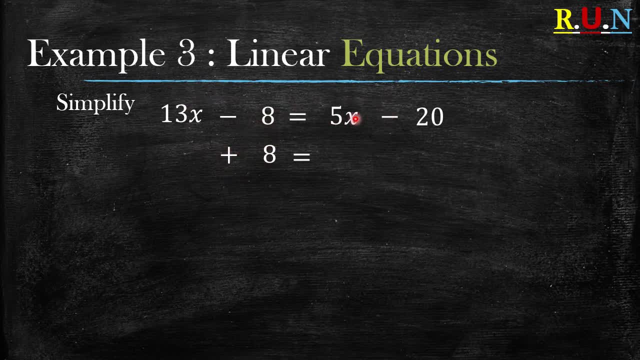 Now remember: whatever you do on this side, you do on the other side. So we plus an 8 on the other side as well. Now remember: when you are plussing the 8, you can't plus the 8 to 5x. 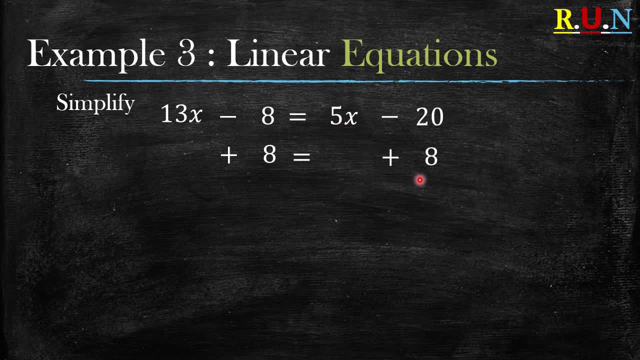 Why? Because 5x is not a like term. But you plus it to the negative 20 because 20 is a like term to 8.. Or in other words, let me just say 20 is just a number And 8 is also just a number without a letter. 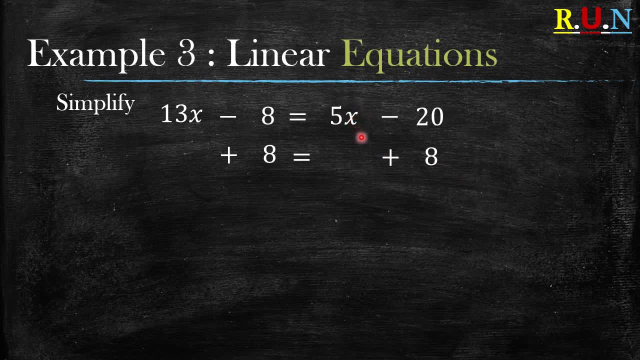 But this 5x is having a letter, okay. That's why when you plus your 8 or your other number, you plus it to the number without a letter. Good. So now when you plus your 8 here, this will cancel out, okay. 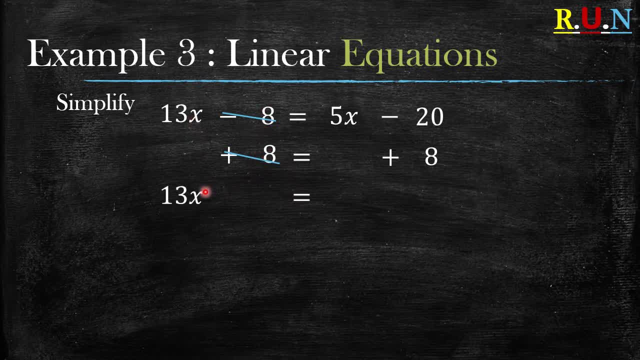 What will be left when you cancel this 2 out? Only 13x. What about on the other side? The 5x will come down the same way it is. And then what? What's negative? 20 plus 8?? It will give you negative 12.. 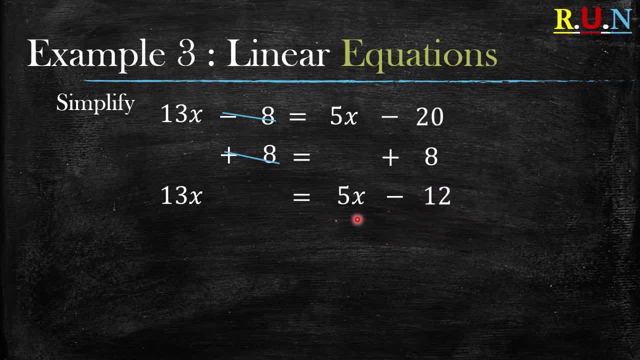 Okay, So now we are left with this 2 on this side, And on the other side, we are left with this 1.. So now, what is our main aim? Our main aim is to have x on one side. 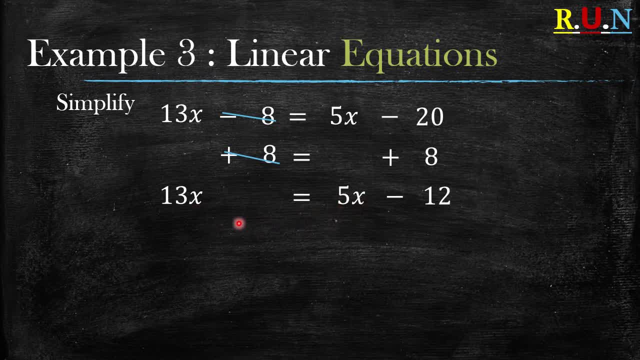 This x variable on one side. So what do we do? Let's look at this 5x. Let's cancel this 5x from here so that we can only have an x on this side. So how do we cancel this 5x? 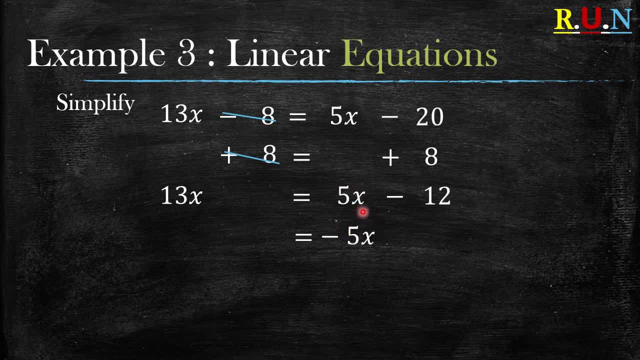 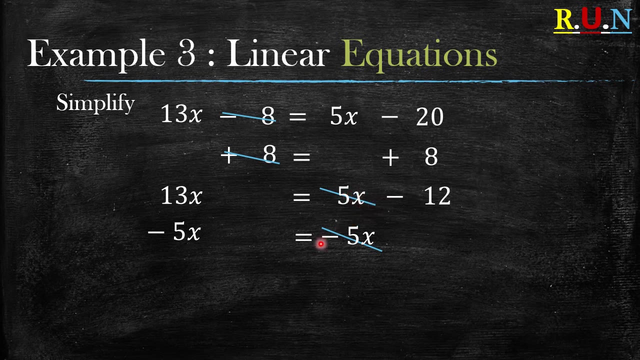 By minusing a 5x on this side. Now remember, guys, whatever you do on one side, you need to do on the other side. So on the other side we minus a 5x as well. So what is 5x minus 5x? 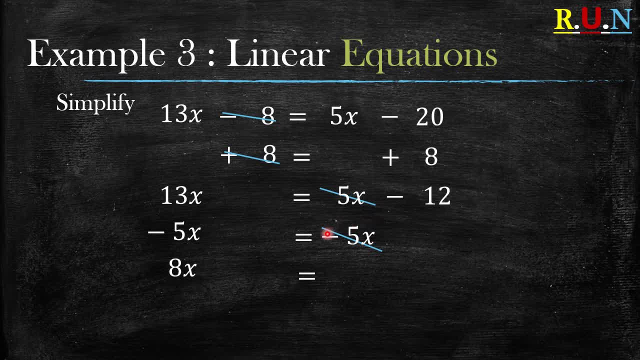 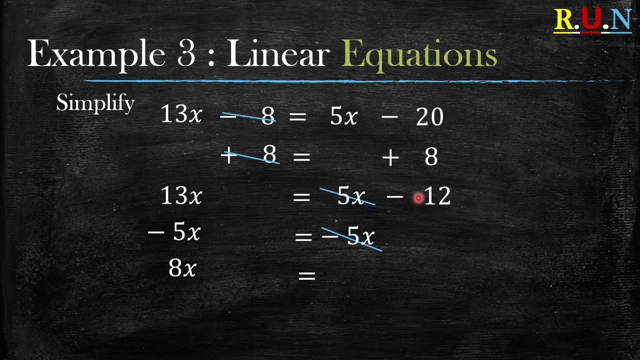 It will cancel out. And what is left? Sorry, On the other side, 13x. 13x minus 5x will give you 8x. Okay, So now here we have 8x After the 5x cancels out. on this side, we are left with negative 12.. 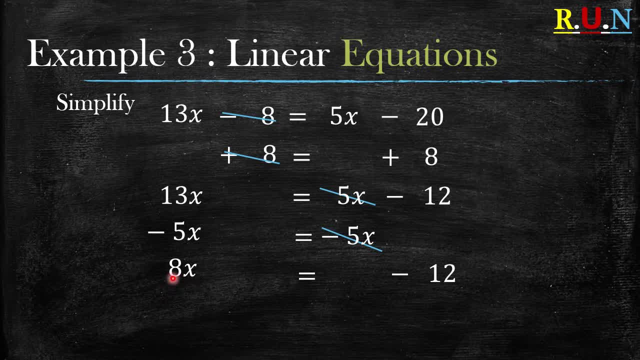 Now 8x. Remember, this is now multiplication. So for us to cancel this out, we need to divide by the same 8.. Now, remember, whatever you do on one side, you do on the other side. So we divide this side also by 8.. 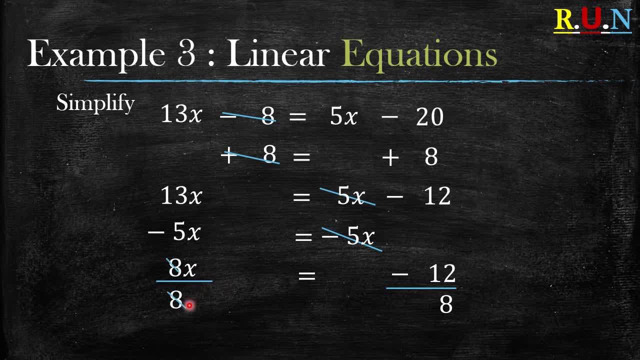 Okay, Now what is 8 divided by 8?? It is equal to x, because these two will cancel out. So the 8 and the 8 cancel out. You get an x only. Now, what is negative 12 divided by 8?? 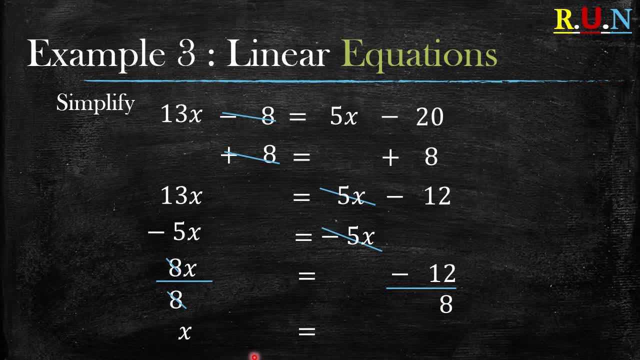 It is equal to negative 1.5.. And just like that, you found your answer. Okay, Thank you all for watching. Please do like, subscribe and share this video And I will see you in the next video. Bye. 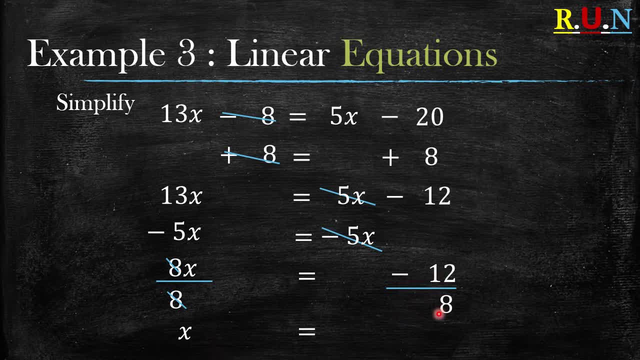 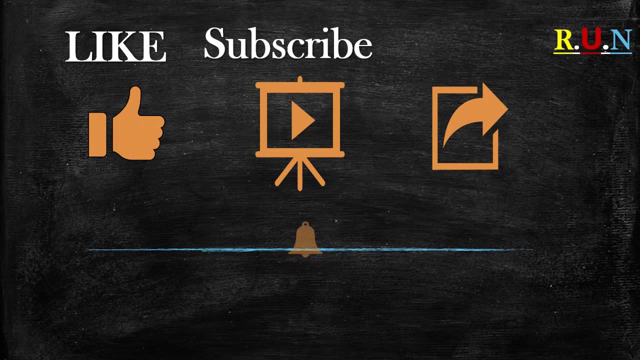 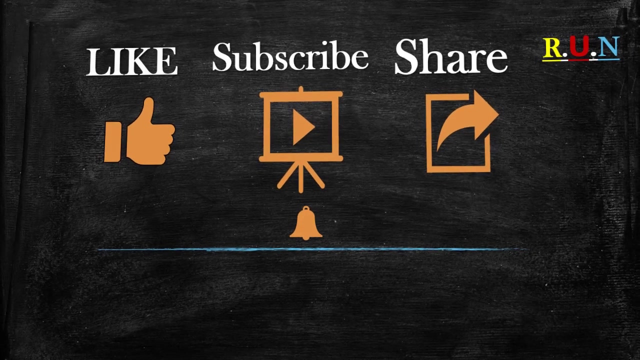